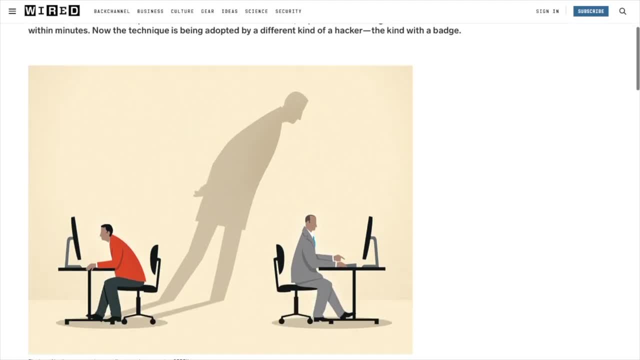 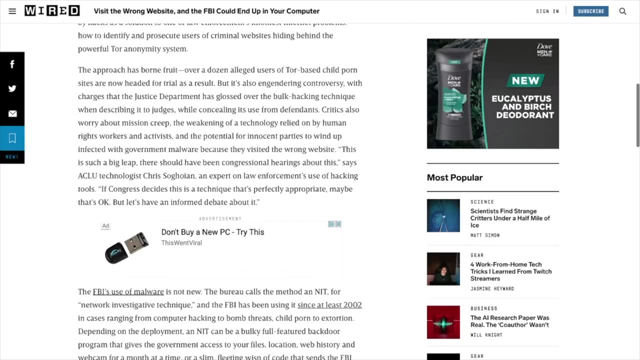 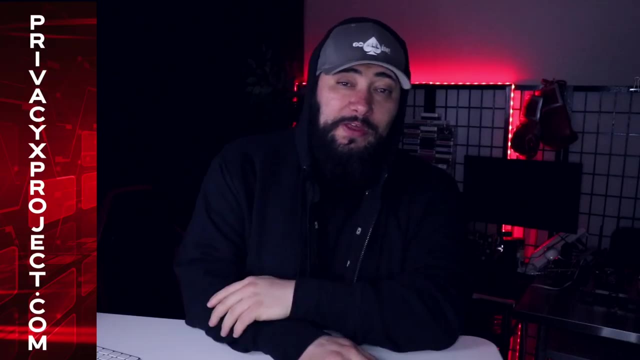 Tor and the FBI and other alphabet letter agencies attacking people using this program. Now, Tor is a phenomenal browser and most of you are familiar how it works. If you're not, I've done videos breaking this down. But do they really put you on a list if you use Tor, That's. 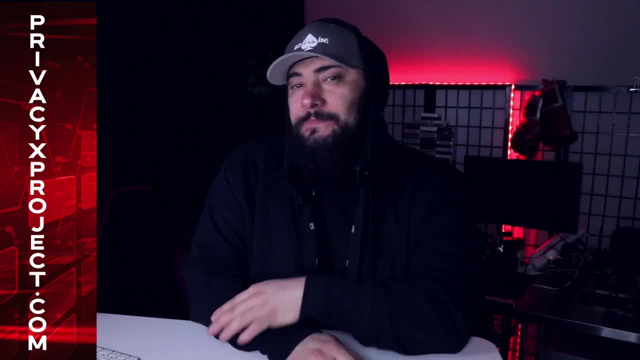 really what we want to talk about. We want to talk about best practices- if you're using the dark web and Tor to maybe stay off these FBI watch lists, but more than that, to make sure you can navigate properly. Now, before we dive into that, I recently just launched the PrivacyX Project podcast. 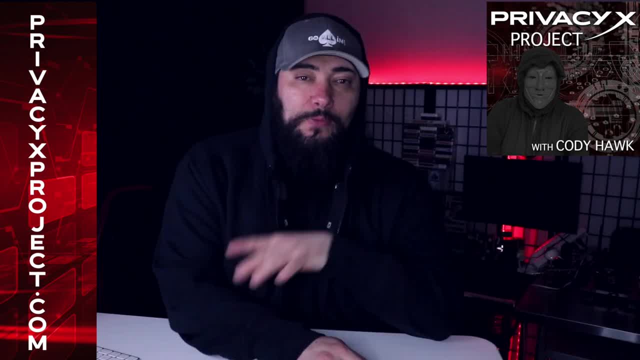 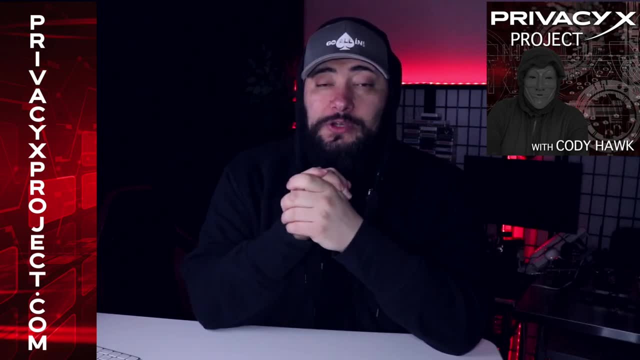 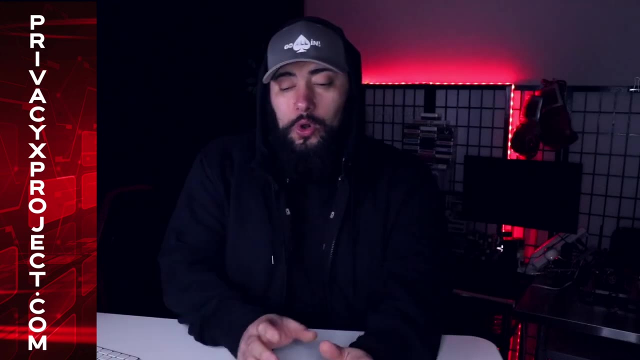 Link will be down below. Check it out. We've got the first couple episodes out. Really excited about the podcast, Putting out daily episodes for the first 30 days to kick it off. So make sure you go to privacyxprojectcom and check out the new podcast. All right, So with Tor. 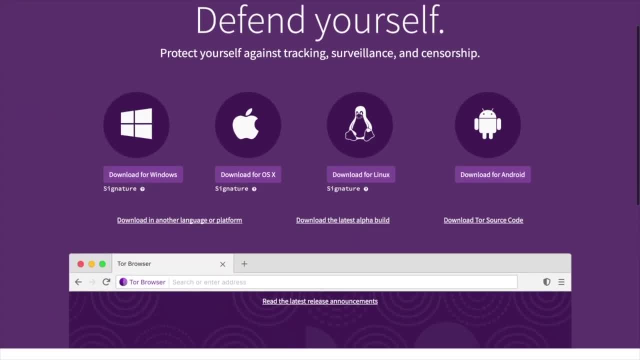 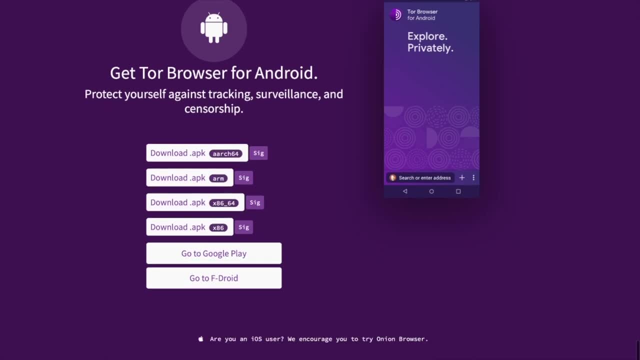 it's a pretty interesting phenomenon. Now, usually, as I've showed before, I will use something like VirtualBox and Hunix, or you can use Ubuntu. You could use something like Cubes, which I'm a big fan of. Basically, you'll have a virtual. 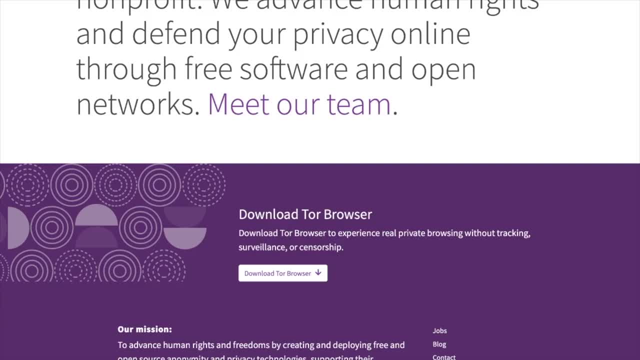 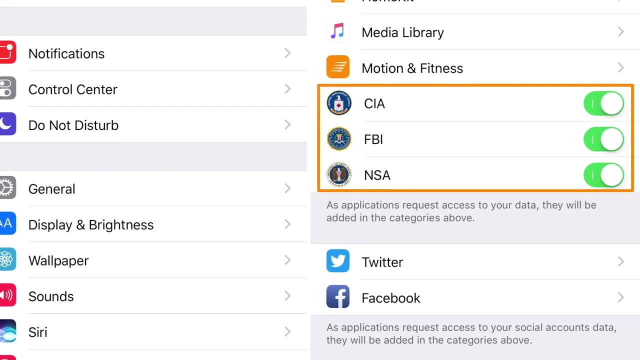 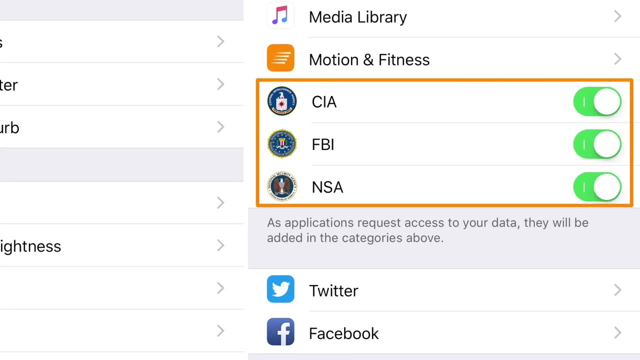 machine for your operating system- Always a good practice. But even on your smartphone, iPhone, or if you have an Android, you could use something like the Onion Browser, or you could use Tor. Now Tor will bounce to multiple different relays, ultimately your exit node. It'll take you. 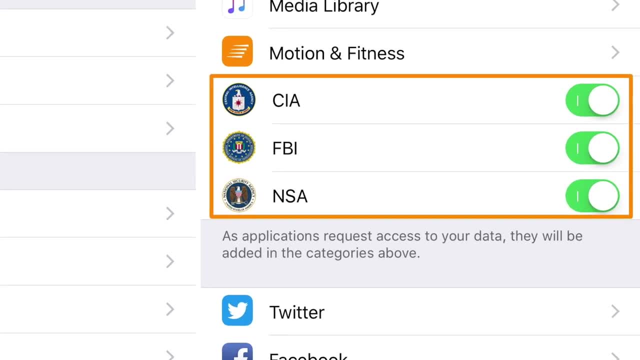 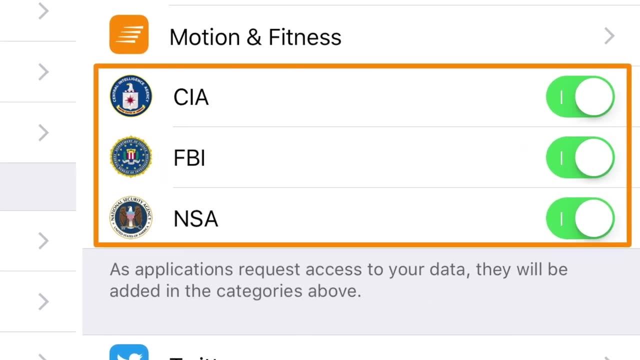 all around the globe in a matter of seconds And it's supposed to anonymize you as a user. And the thing with Tor is more and more people have been using it- Millions of people over the last several years has really helped hide in plain sight And that's the fundamental feature that adds. 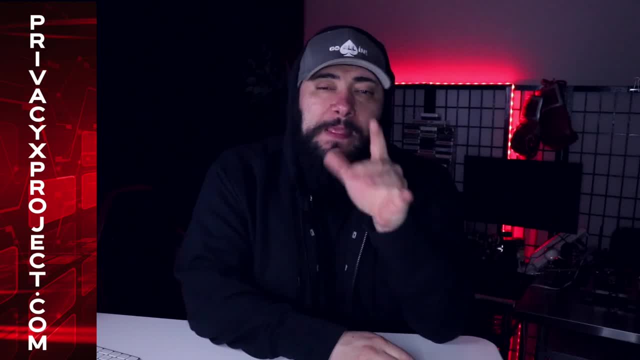 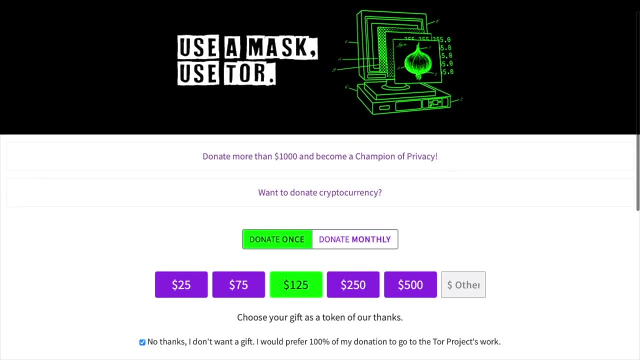 the most value is the ability to hide in plain sight and the ability to be able to be an anonymous user. Now the FBI and the other alphabet agencies have known about this for a long time and they've been trying to crack the code. There's been talk. 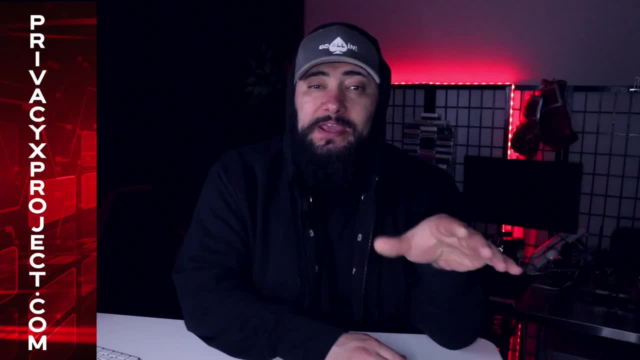 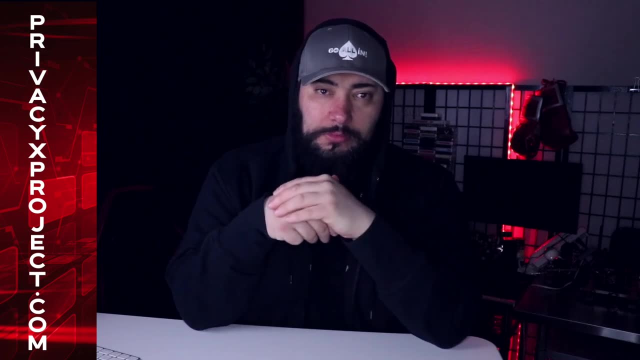 there's been talk that they have not. Obviously, they're going to put out information to make you think that they could do more than they can do in this scenario, But really it doesn't come down to using Tor. It's not illegal. It's not illegal to go on onion or the deep web. What's illegal is if. 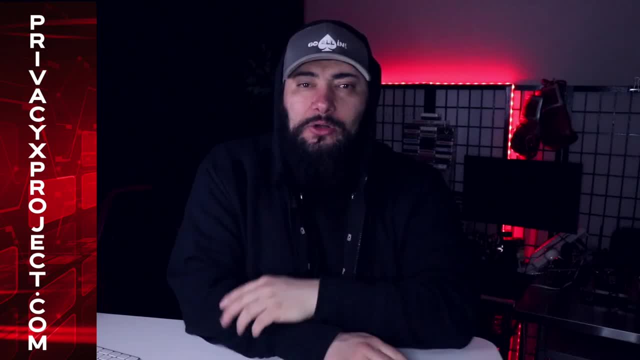 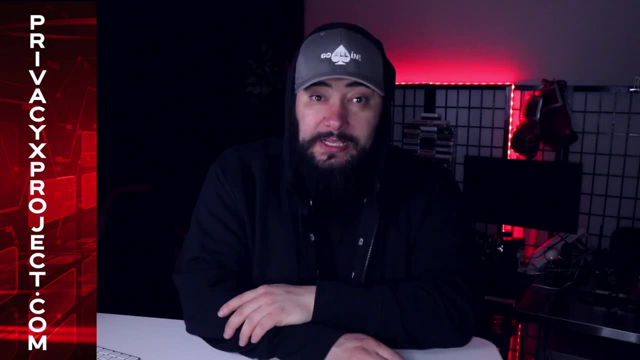 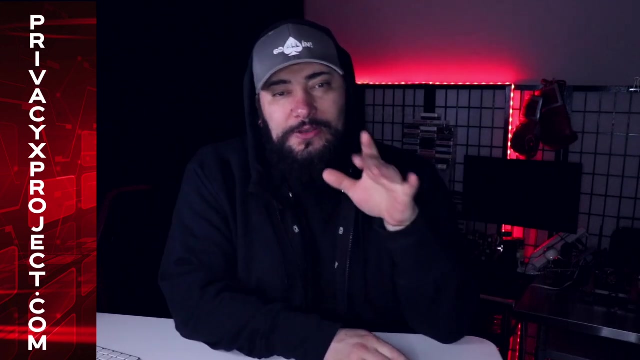 you take action on some of these illegal websites. So I think the FBI could probably track many of these sites, And I think they probably do for good reason. You've seen things like Silk Road, which got shut down years ago, Dread, Pirate Roberts- You've seen the things come out with all the illegal 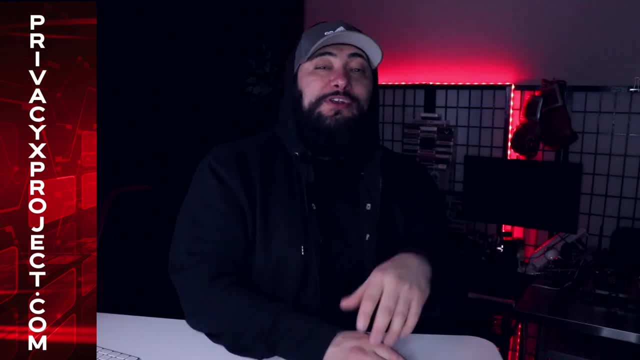 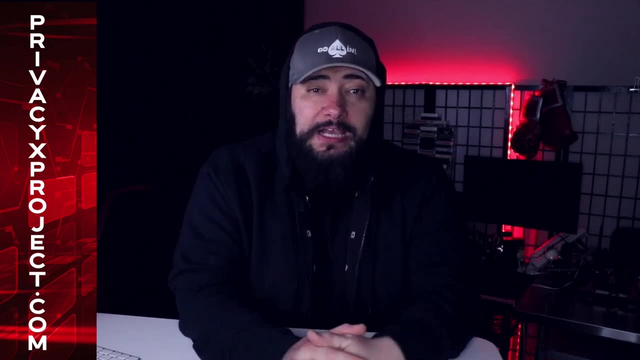 activity that can be found on the dark web. I do not recommend you have your kids go on the dark web, but using it for anonymity purposes might be a good idea, because we're at a crossroad. On one side, we've got Tor. On the other side, we've got big tech, big data, big brother spying on every. 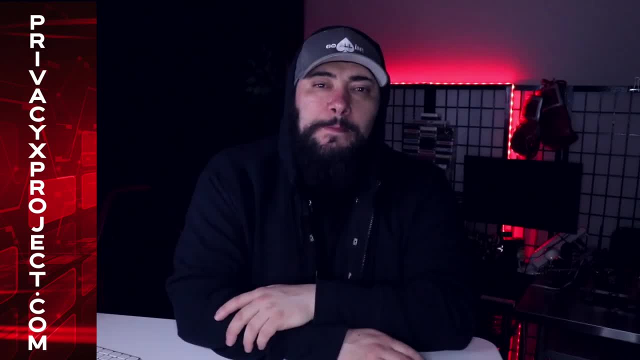 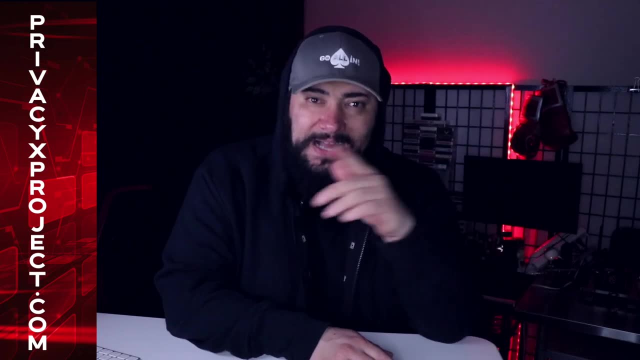 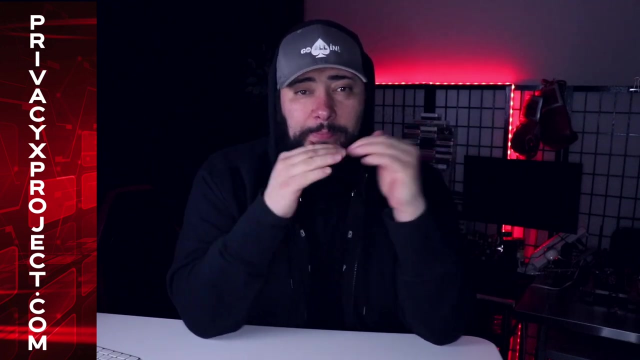 single thing we do, from our devices to our personal computers. And if, if this is a scenario where we've got to pick a side, well, going for your privacy and anonymity is always a great option, But you need to keep in mind when you're going through this process: you want to not overstep the bounds. 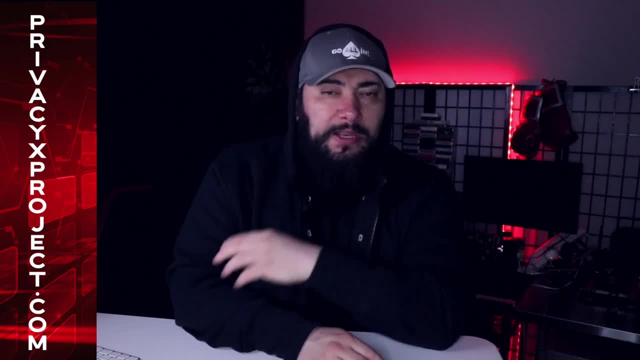 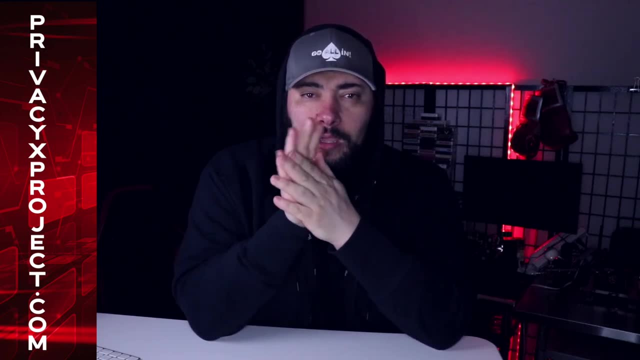 Now, if you use a VPN, which I've talked about, I use ProtonVPN and Private Internet Access VPN. No, I'm not an affiliate, I'm just a happy customer. But if you use a VPN, get onto Tor. You're trying to anonymize. 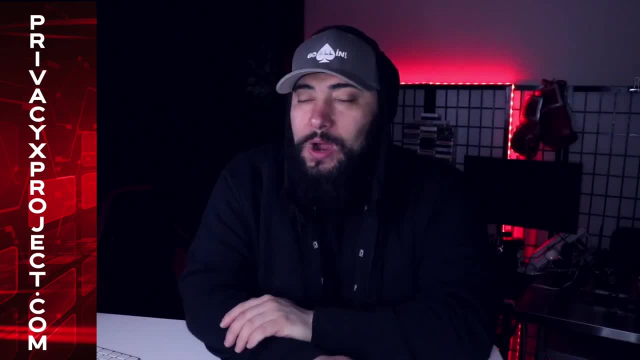 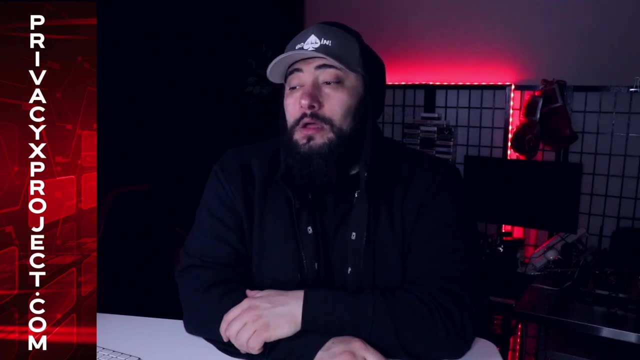 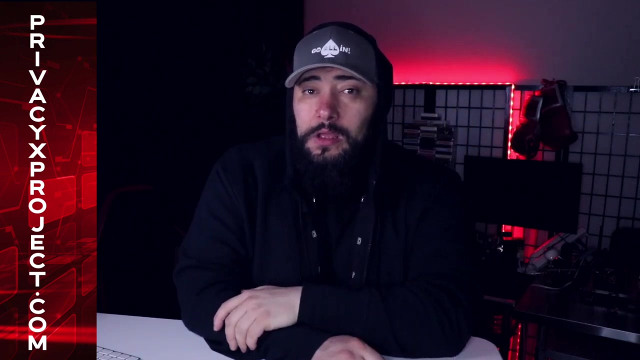 Bloomberg pal, You're trying to to have an anonymous IP address, then going through Tor, then you're in a pretty good place. Now, ideally, if you're using a virtual machine like VirtualBox and then using something like Hoonix. 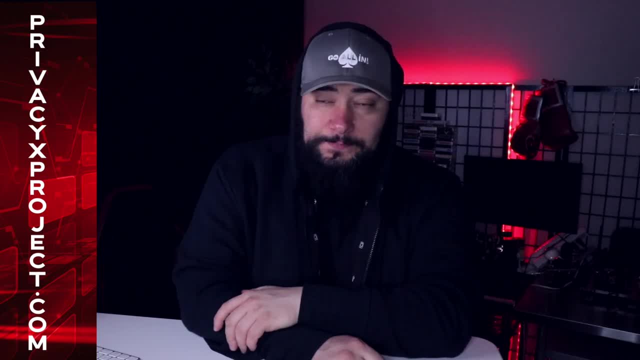 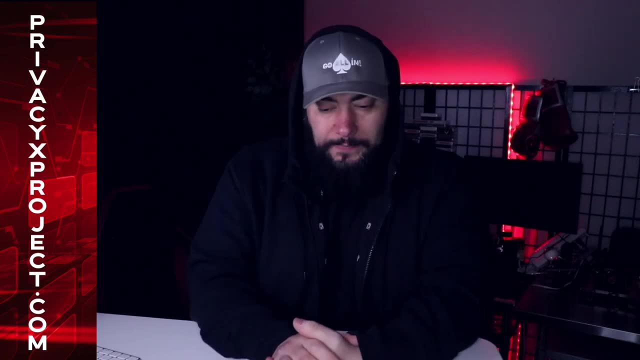 or like Cubes or one of these other OSs, then you potentially could be in a pretty safe space. Now keep in mind: all of this is for your anonymity, not so much to do anything nefarious or illegal. I don't recommend doing anything illegal. 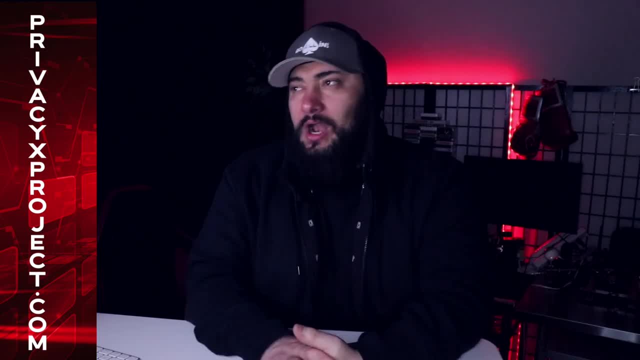 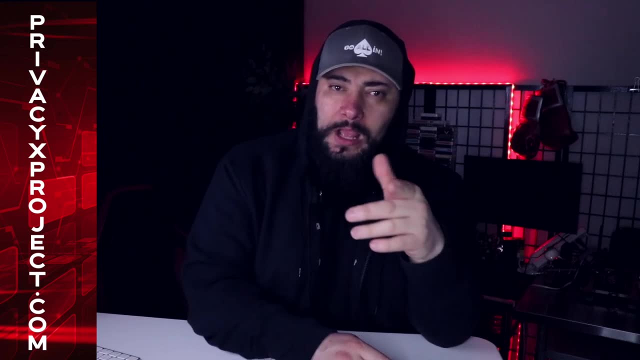 on the internet or otherwise. So if you're trying to commit crimes, there's a lot of people on there and what happens is it's not just about committing a crime, it's about wrong place, wrong time, And that's part of the problem with Tor. 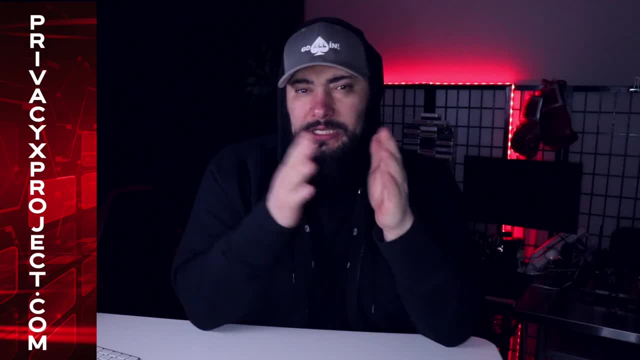 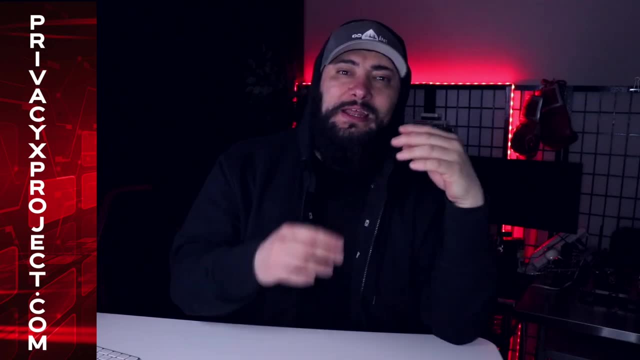 and so you really gotta watch the way that some of these sites will attack you, because the FBI has seen a lot of people go through these different scams. You can go to a website, click on something- it is a cloned website. then you've downloaded something on your computer. 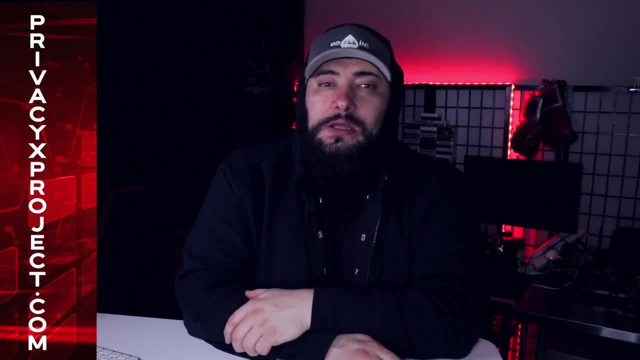 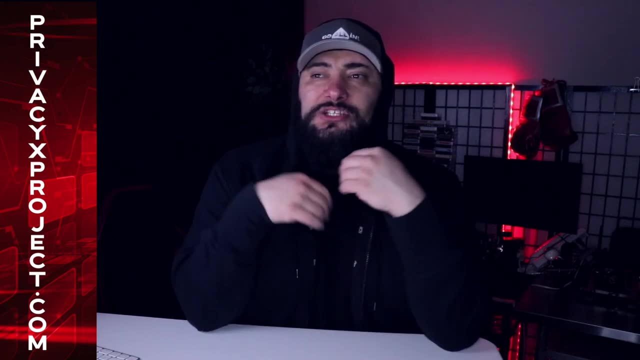 and the FBI shows up knocking on your door because you downloaded some illegal stuff to your computer. but you just thought you were on a regular website that you go to all the time, And so that's really where you gotta be careful. and if somebody backtracks you from an exit node like Tor, 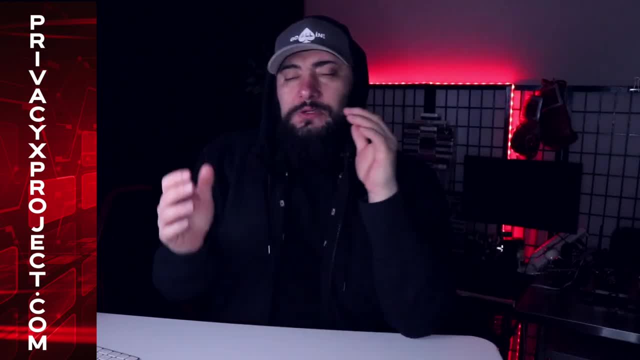 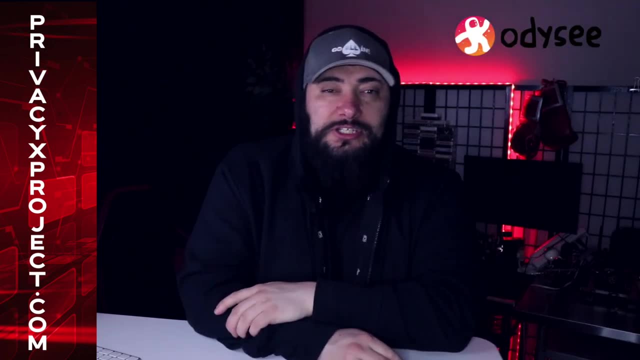 can they? What can they do? Can they get to you? So, as we start to pivot into the blockchain technology, if you haven't already, make sure you follow me over on Odyssey. Odyssey's incredible Been growing slowly but surely over there. 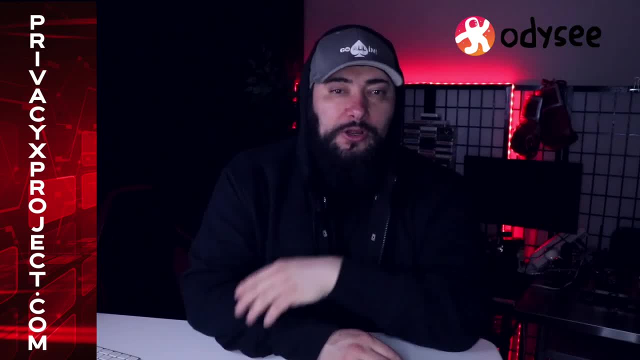 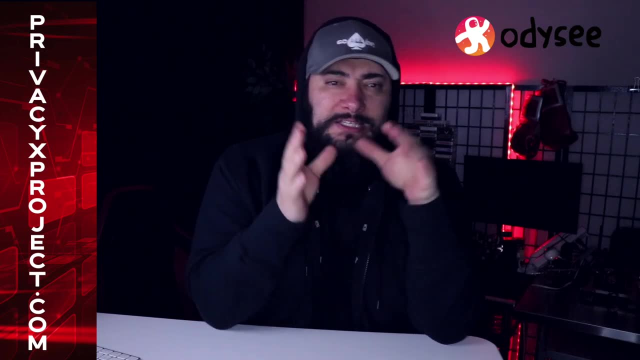 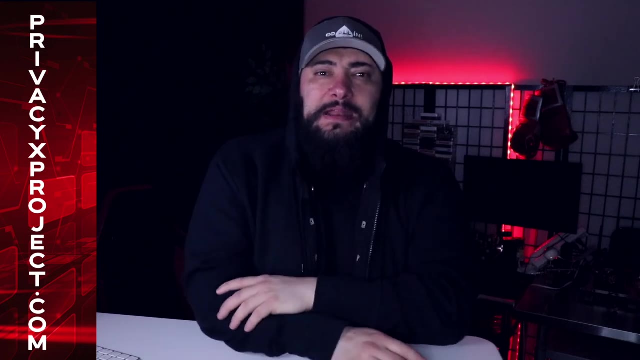 And I love the idea that they have a library of coin or library credits, Starting to decentralize. I think eventually Tor will start to go to the wayside a little bit, because it's been so heavily monitored and investigated by agencies with the alphabet letters in front of their name. 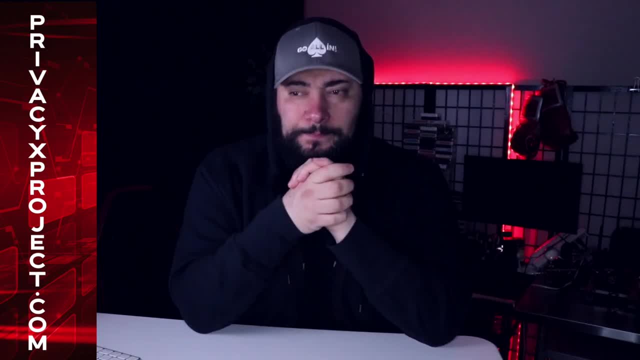 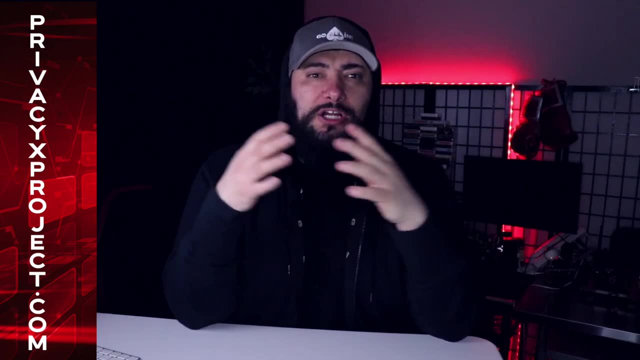 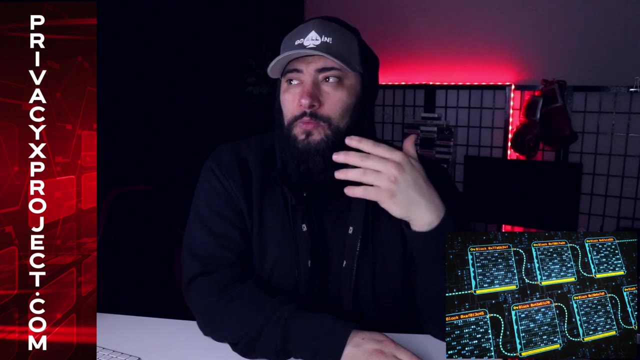 But I think, as we go more decentralized, as we go more blockchain, as we try to anonymize sites and addresses and owners- similar to how you try to anonymize your blockchain wallet, which, if you keep it private potential, or as we have more privacy features like Monero- 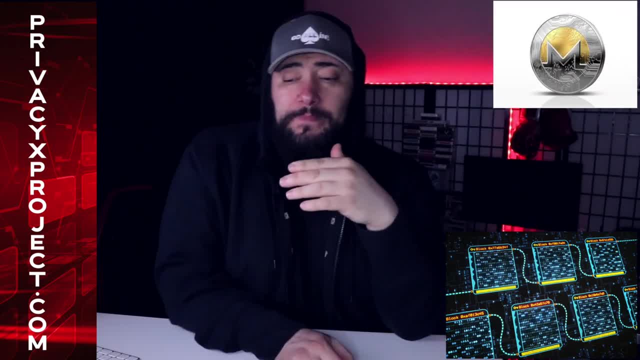 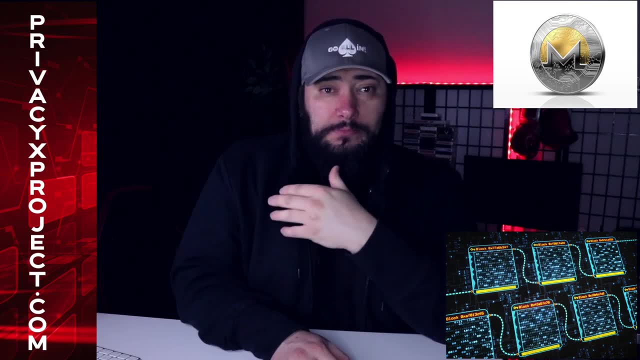 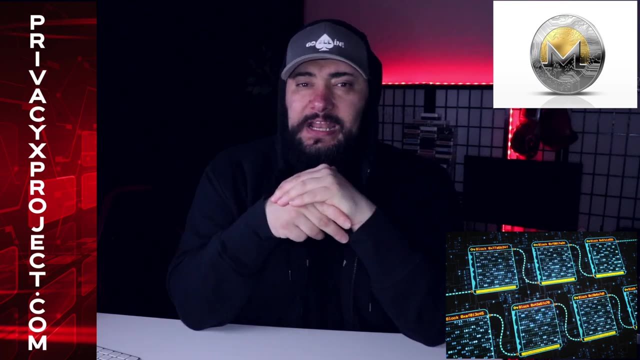 one of the better privacy coins. as we see this technology shift into the core OS of using the internet- not just the operating system but your operating experience, how you navigate through the web. I think that's gonna help give you some possibilities for privacy. 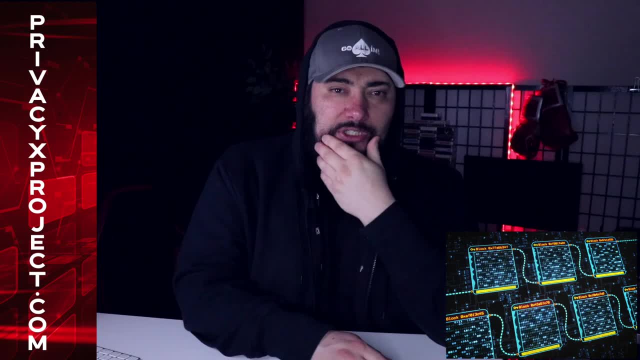 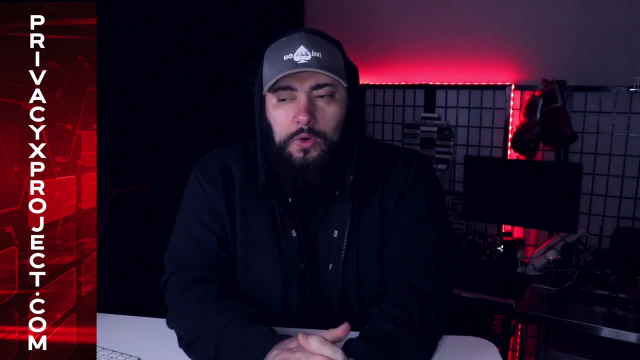 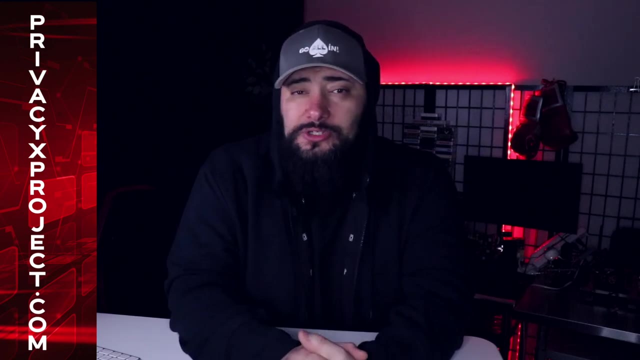 On the other side, you've gotta be careful that you're not setting up a structure that is monitored, that is being scanned. So with Tor, right now, Tor is one of the best tools to be able to surf the web anonymously, And that's why a lot of people are trying to crack the code. 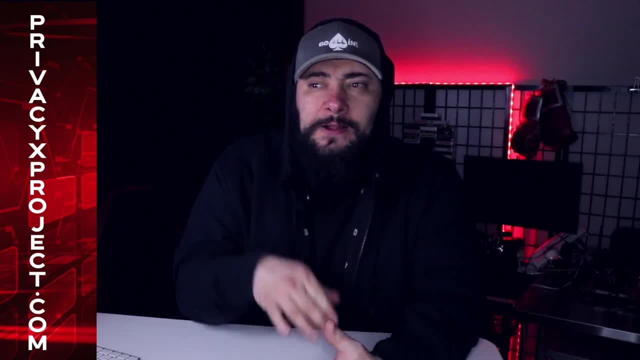 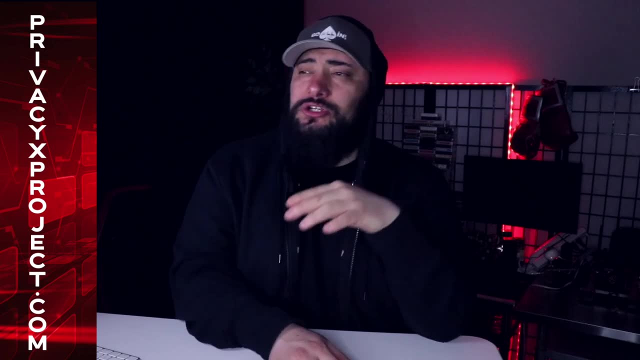 Now Tor has some very practical value in other countries where things can be blocked, or for journalists. but in a scenario like what we've seen a lot, with the FBI trying to track, they're trying to track users And people say, well, what if they put me on a list? 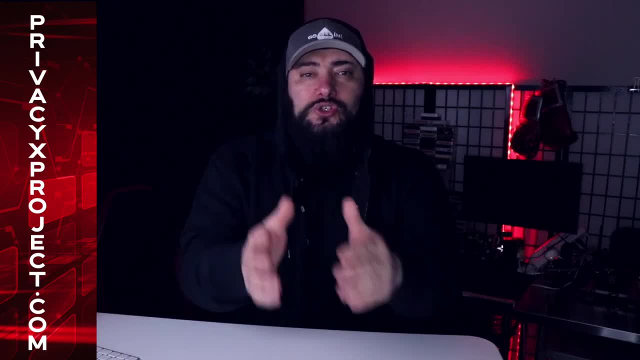 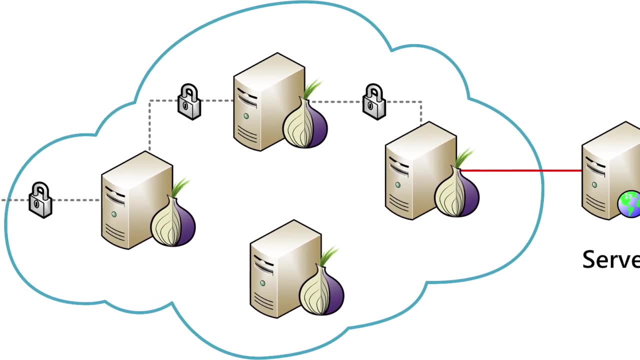 Well, here's the problem: When Tor has millions and millions of people using Tor, what list right? What list are they gonna put you on? A list of 20 million people? You know, when Edward Snowden released it, the government was virtually spying on everyone. 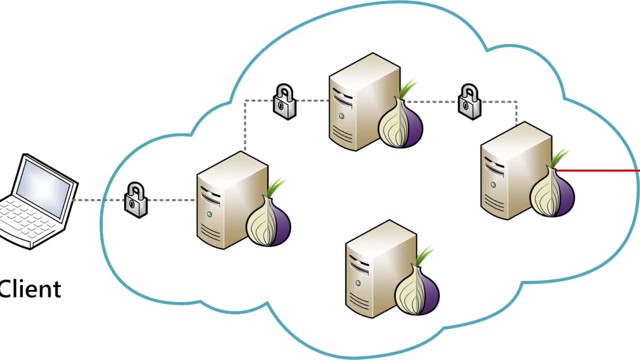 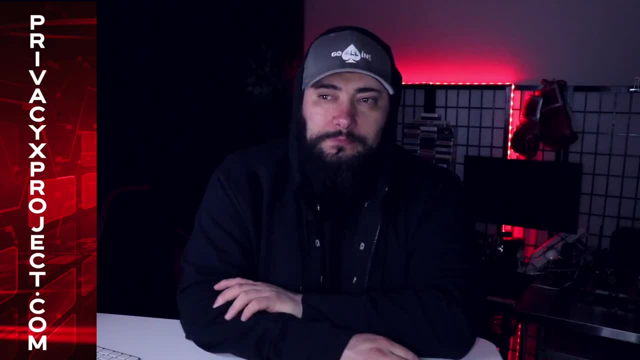 Well then, they have the ability to take action against no one. So again, you're hiding a plain sight. And so if Tor had 200,000 users, then it might be possible For the government to put all them on a list. 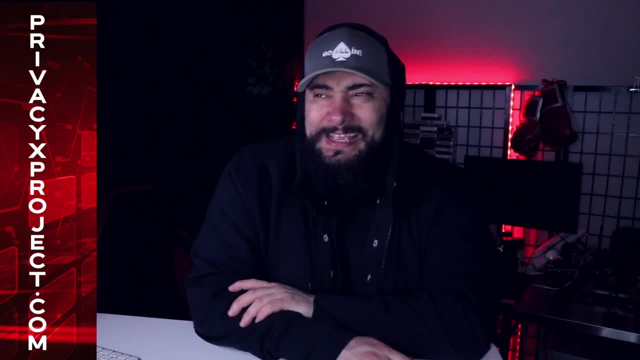 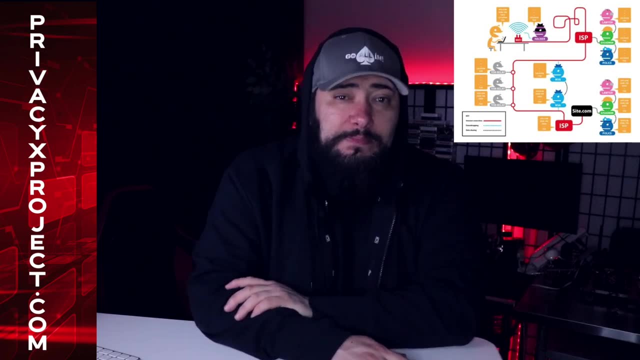 and try to allocate some resources to categorize that list into the highest potential threats. But now that Tor has become more mainstream and millions and millions and millions of people are using it- it's talked about all the time, every day, And people are using it just for their regular browser. 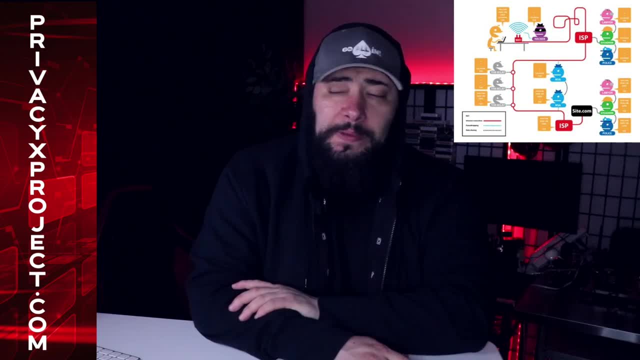 You got the onion browser on iOS, you got Tor on Android, and people are using it both on mobile and on desktop platforms. The application can cross platforms. You can cross platform on all your devices. Well then, it makes it a lot tougher. 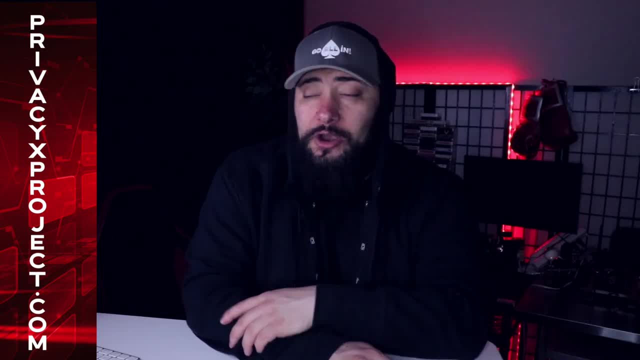 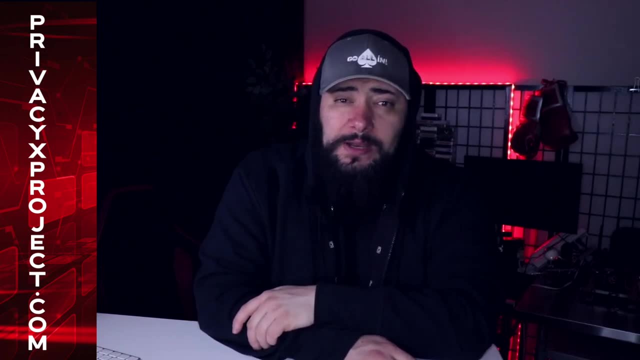 as Tor has their own small piece of the market share, And while they only have a small fraction of the browser market, a small fraction of the browser market is still extremely hard to track when you have a list of millions and millions of people, And so you become hidden in plain sight. 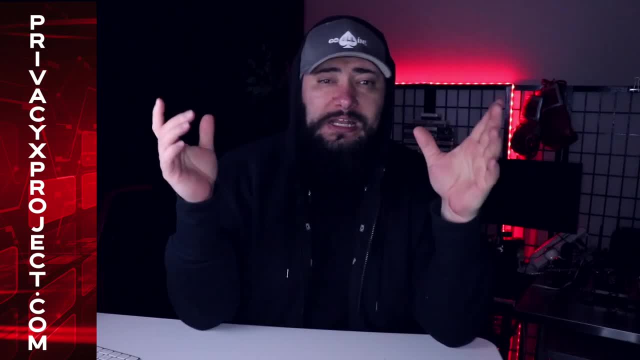 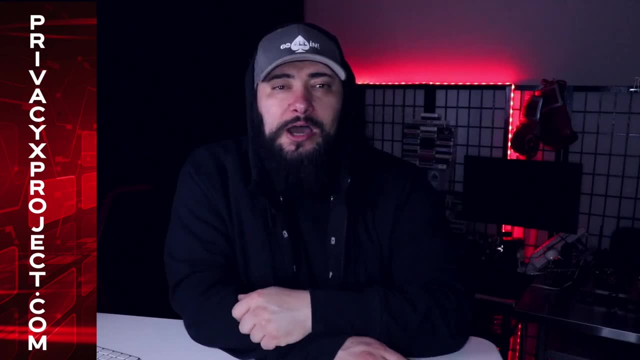 So, yes, if you're doing illegal and nefarious activities, Tor does not make you a ghost- You will get caught. Lots of people have been caught off Tor, But these lists- you're probably on a hundred different lists. We live in a world where all's the government does. 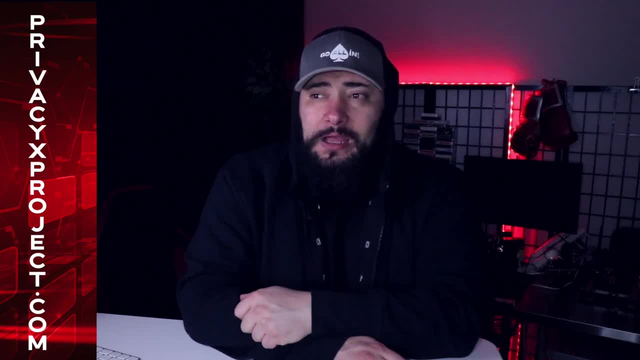 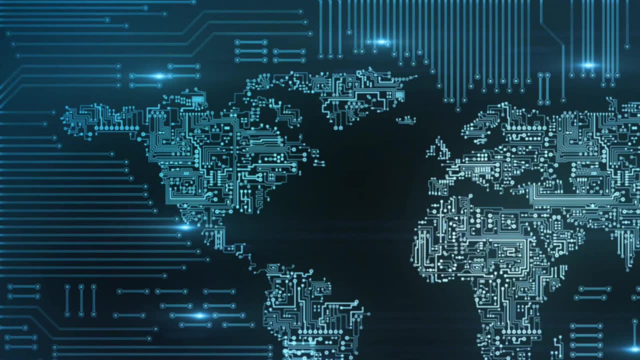 and all's big tech and big data do is categorize everything you do, everything you say, all the actions you take, all the interests, hobbies, all your thoughts. I mean you literally type your thoughts into Google and they categorize your thoughts. 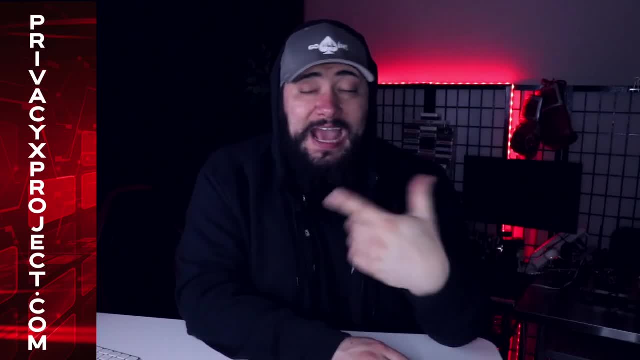 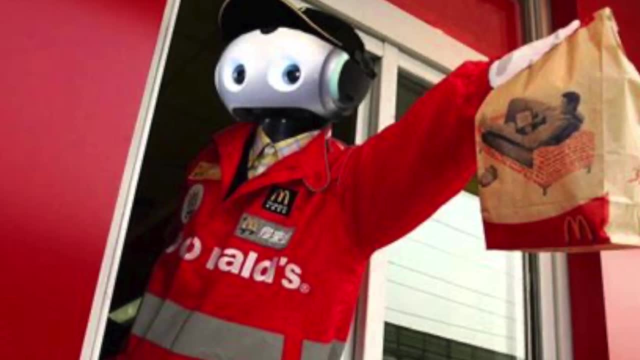 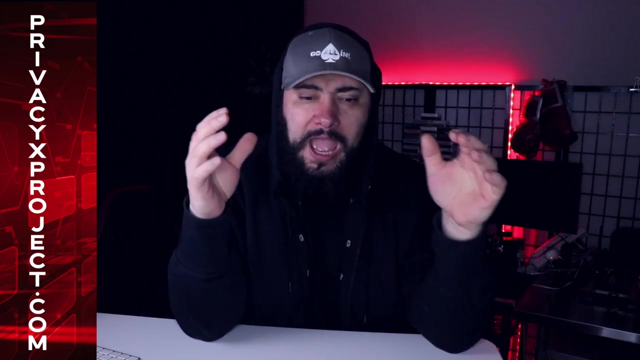 They catalog your thoughts. It's connected to an IP address And even if it's not, machine learning has gotten so good already, even though it's not very impressive yet, but it's gotten good to the point where they can. they've got algorithms that can take your behavior. 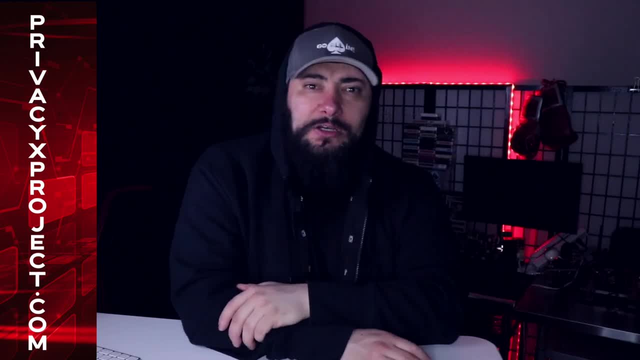 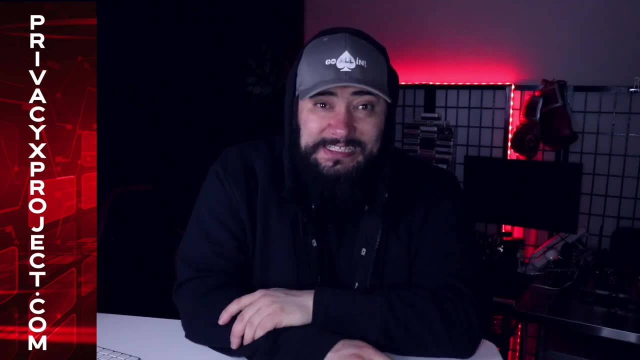 and narrow it down based on the consistency of your behavior. And this is the problem that a lot of people don't understand is they don't have to get directly to you. They could get a guess that is right 99% of the time, based on the things you do.